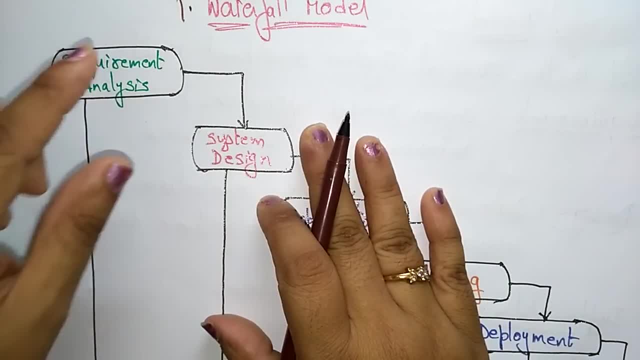 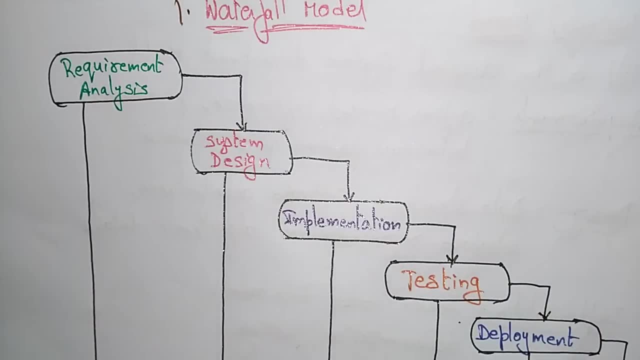 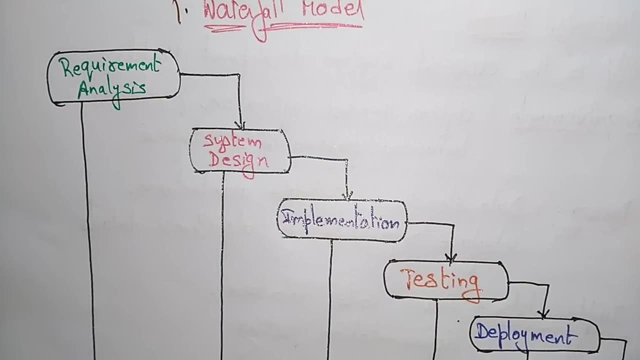 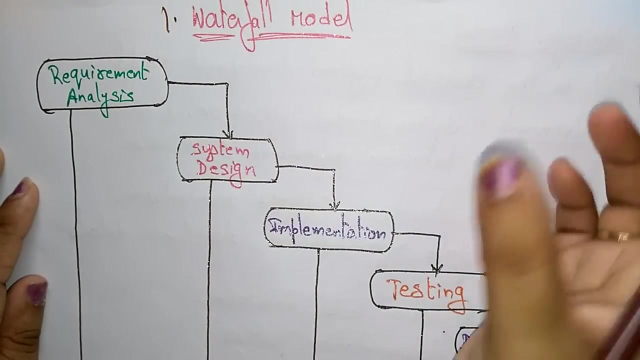 So the waterfall model, this is the first software development lifecycle model to be used widely in software engineering to ensure success of the project. So almost all the software engineers are used to use this waterfall model. So in the approach the whole process of software development is divided into separate phases. Suppose, if any process is there, if any product is there, if any problem is there, that problem is divided into two phases. 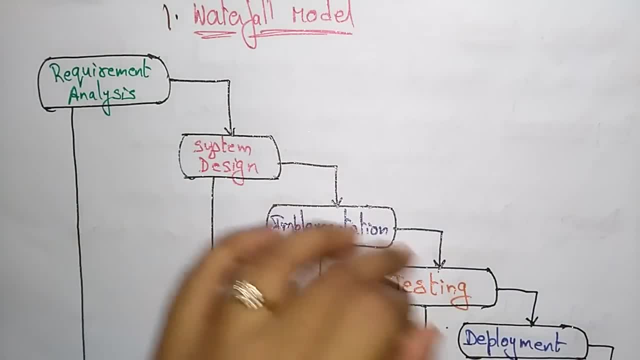 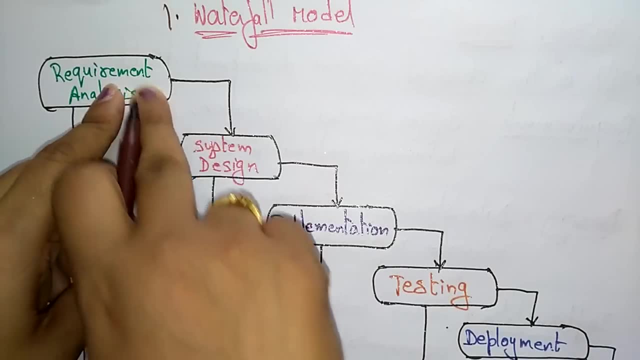 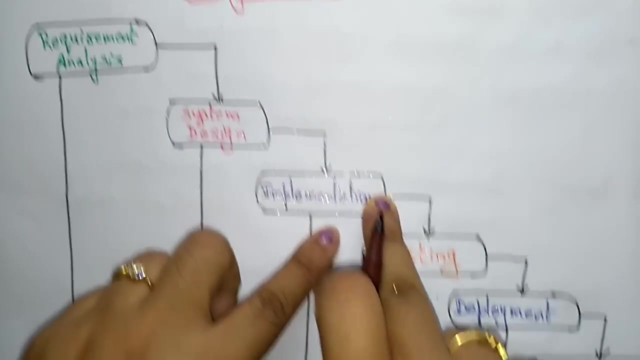 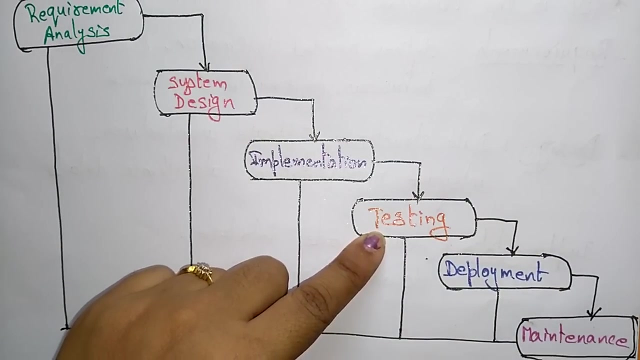 So the waterfall model is divided into series of phases, different phases. Here the outcome of one phase acts as an input to the other phase. The outcome of requirement analysis acts to the input. Outcome of system design, input to implementation. Outcome of implementation is input to testing. Testing is deployment. Outcome of deployment is maintenance And it is input to the maintenance. This is outcome of one phase is access and input for the next phase. That should be included. 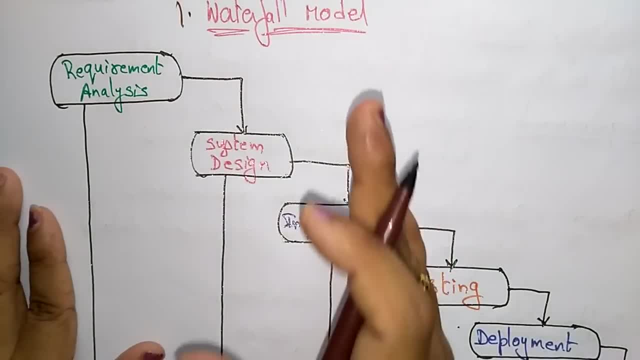 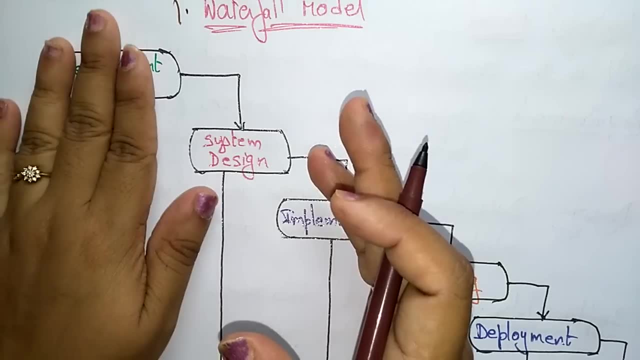 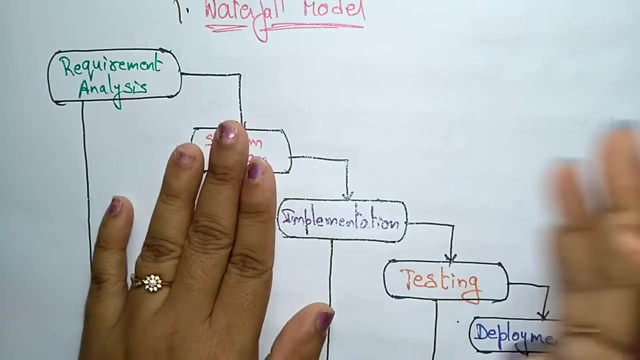 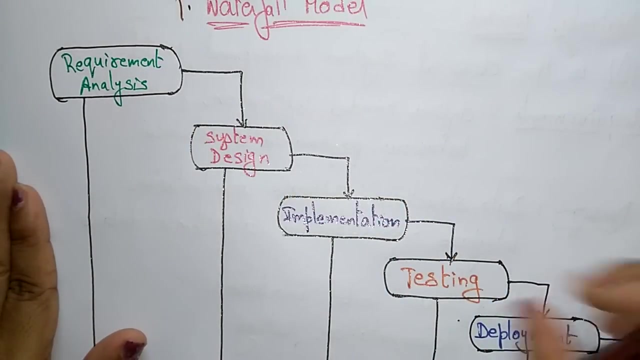 So it is a nice this. So here you are, approaching in sequential. Now let us see. And one thing you have to remember: that once, if one phase is completed, then only you go for the next phase Without the completion of the first before phase. you are not supposed to go for the next phase Once it is freeze, next go for the next phase. Once it is freeze, next go for the next phase. Like that we have to follow it. So that's where we call it as a waterfall model: Water first drop, here It next it comes to next stage, Next. 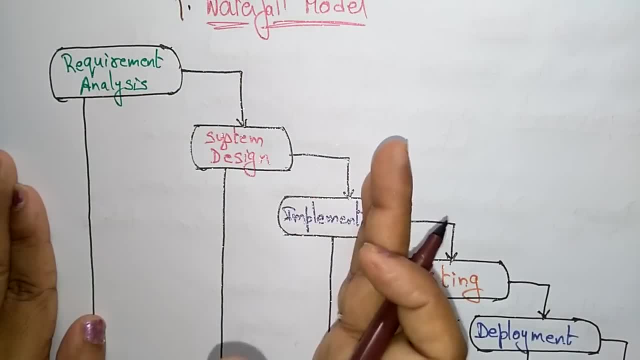 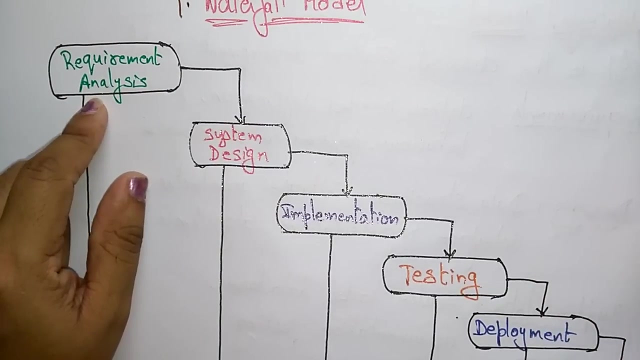 course to change Wang stage. if you drop the water, the stages will be changing from high to low whenever we are pouring a water from terrors. so first it reaching first day, fifth floor, next fourth, next third. like that it is coming down, so like that it has to follow, like that. now, first, see the requirement analysis. 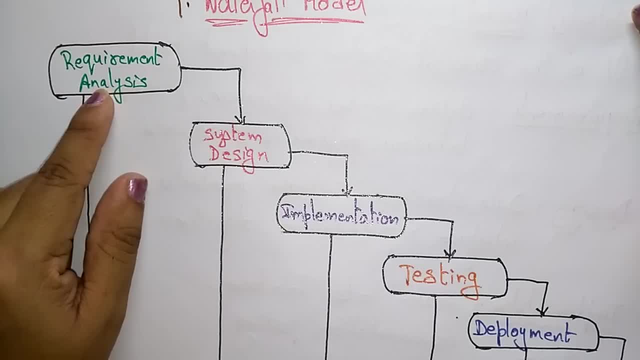 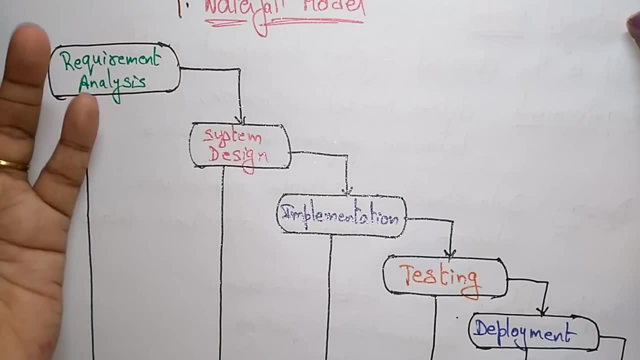 what do you mean by this requirement analysis? so here the requirement gathered and documented in a requirement specification document, so whatever the user's requirements, suppose i am saying to the person- means i want these are the specifications, i need the output like this, i want the product like this. i am going to run an app like this. so you are giving some. 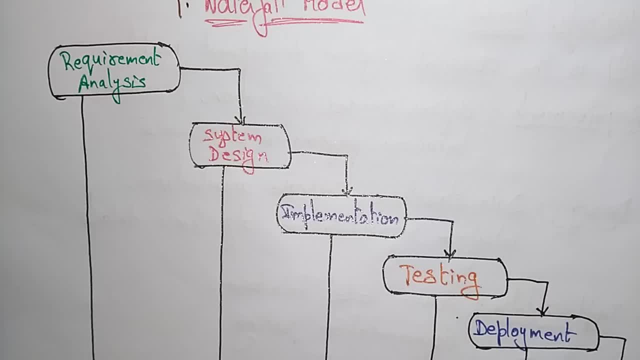 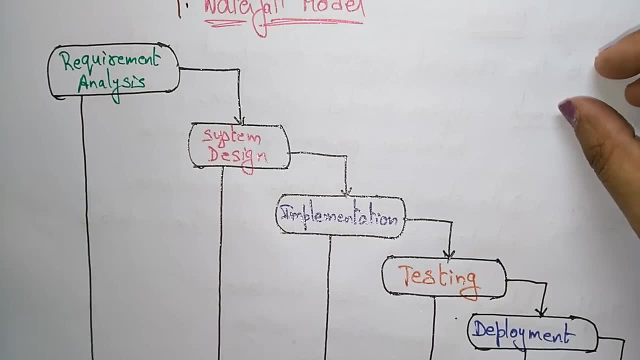 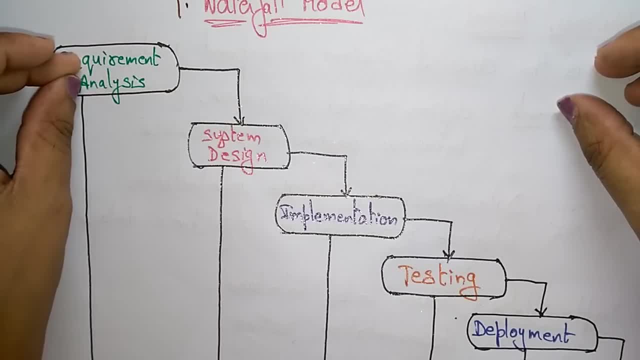 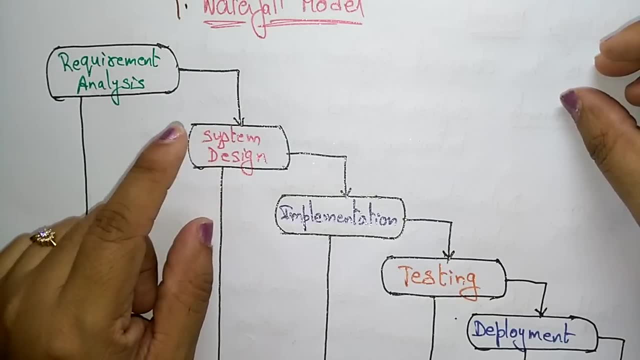 are the customer requirements that will be first documented. after that the system design. the system design helps in specifying uh hardware and the system requirements and also defining overall system architecture means what type of hardware we have to use and whatever the requirements that system requirements that we need, and also defining overall system architecture to 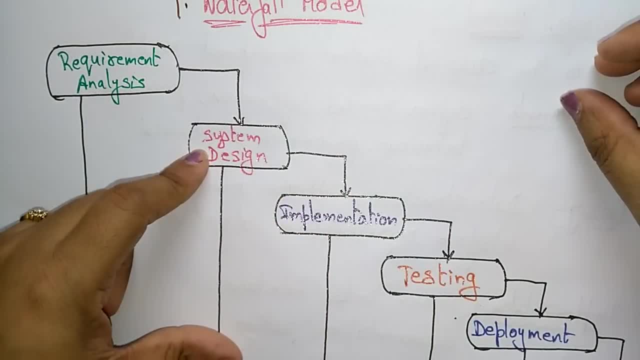 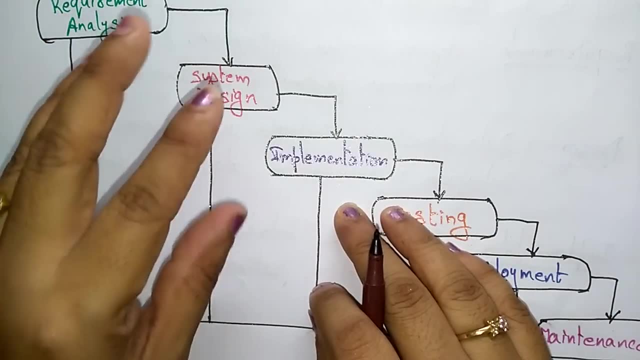 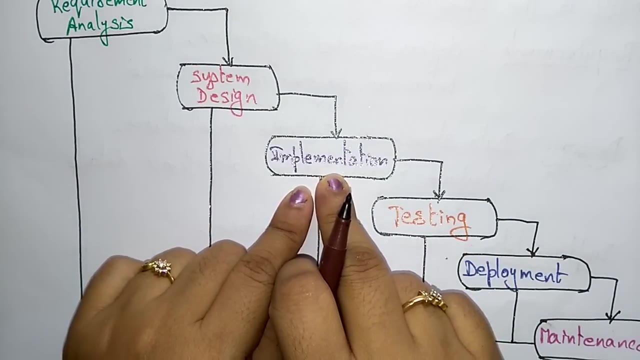 develop a complete system, whatever, whatever they need. that you call it as a system design. so that will be designing in this phase. okay, i know the documentation. i had seen the hardware components also. next they go for the implementation. so in the implementation, with input from system design. so whatever the input that we are taking from the system design, the system is developed in. 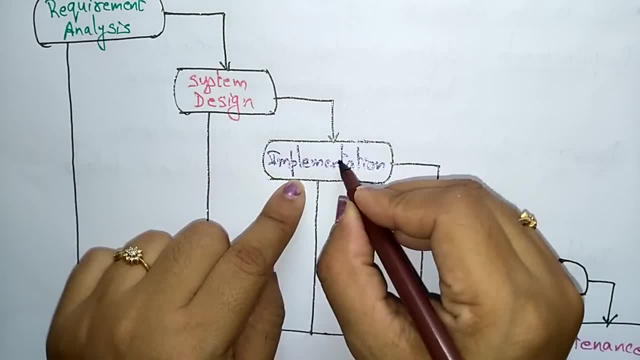 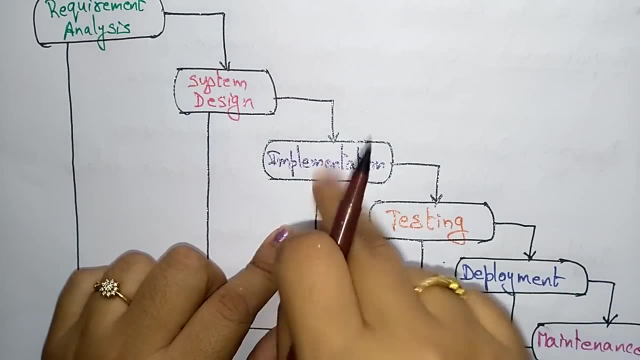 small programs called units. so here we are implementing the program into small units. okay, so here each unit is tested for its performance. so here we are implementing the program into small units. okay, so here each unit is tested for its functionality and it's referred as unit. testing means we are writing a code and we are testing. 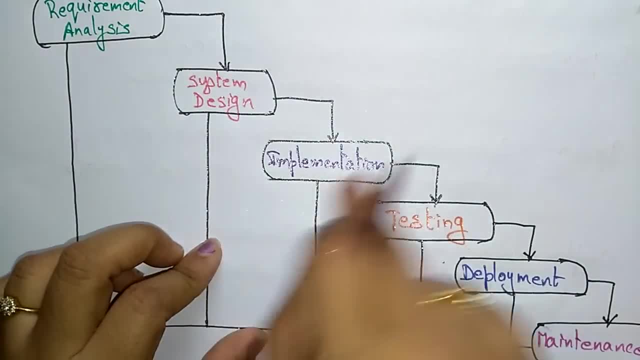 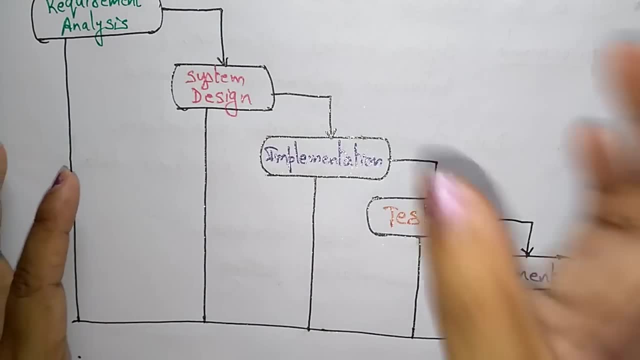 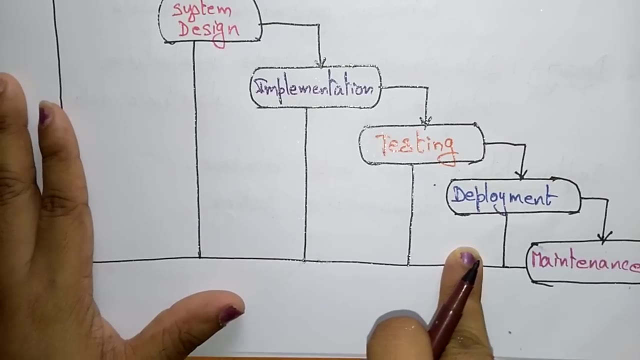 that each unit, by using unit testing, so that everything will be coming under the implementation. okay, my product is over and it is every unit. small programs are tested and it is successful. so that will be checking in this testing after that deployment. okay, so in testing, and here you can also call it as integration and testing, let me 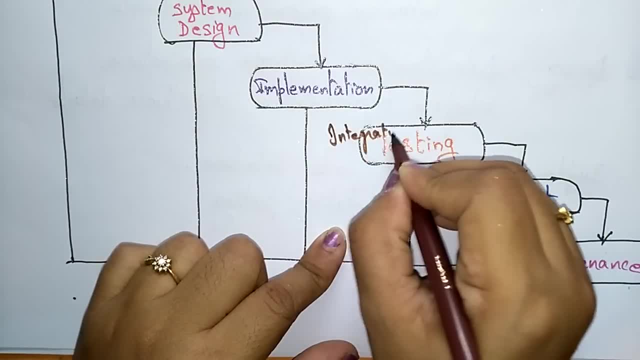 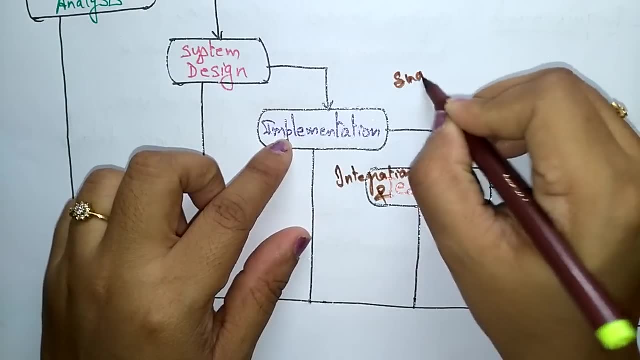 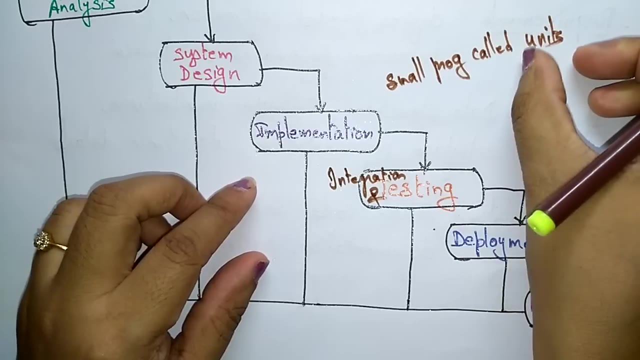 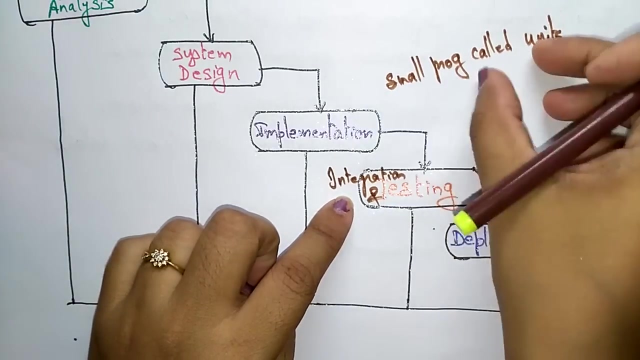 testing and here you can also call it as integration and testing. let me write one more point: integration, integration and testing. so here i'm making the program small programs, small programs called unit units. so each unit we are testing. so after that you have to combine all units that you call it as integration, all units are integrated and test complete product. 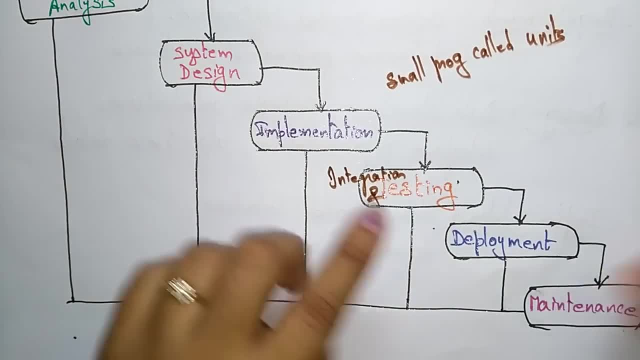 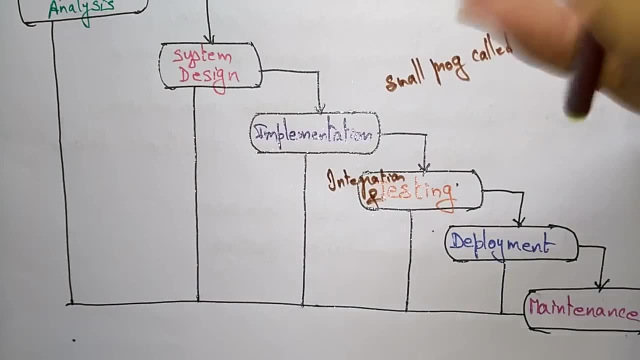 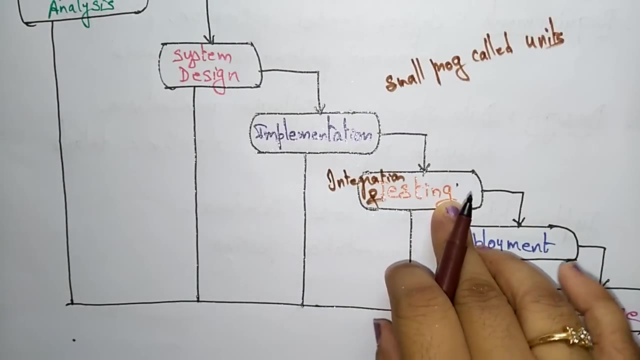 for any faults and failures in this phase. so next they come for the deployment. deployment is nothing but once the functional and non-functional testing is done- okay, everything was done. the testing and the functional, non-functional, everything is done. okay, my product is completely fit. then you are ready to deliver the product to the customer environment or you directly. 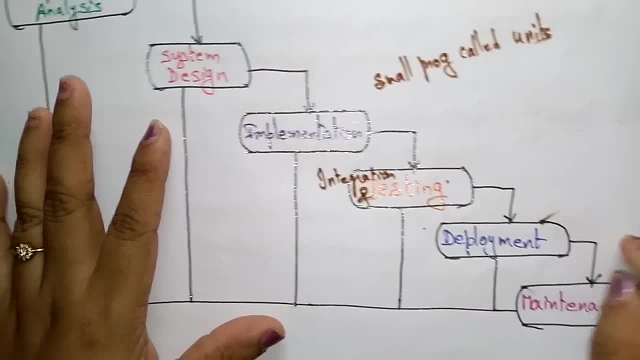 releasing into the market. that stage you call it as deployment. okay, i released everything and my product is ready to be delivered to the customer environment. so you are ready to deliver the product to the customer environment. so you are ready to deliver the product to the customer environment. 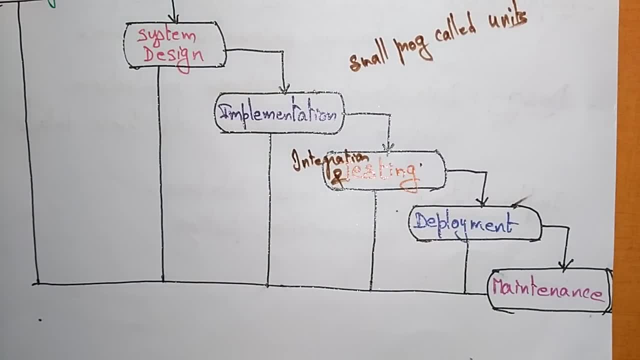 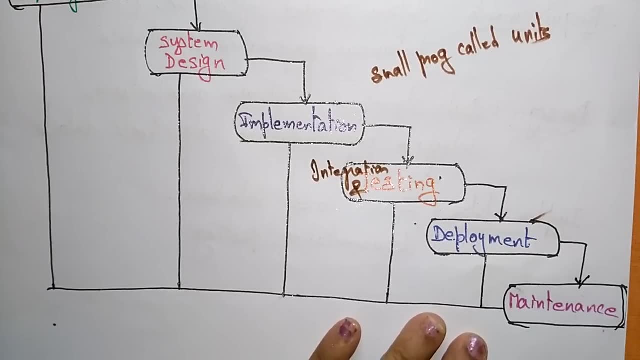 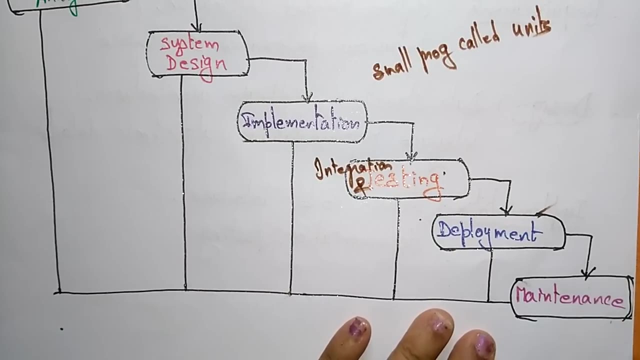 now running in the market and my customer is using. so, even though if your project is over, your product was delivered. if any issues come up from the client environment, you have to be fix those problems and also if they want any enhancement to that product, you have to add that. 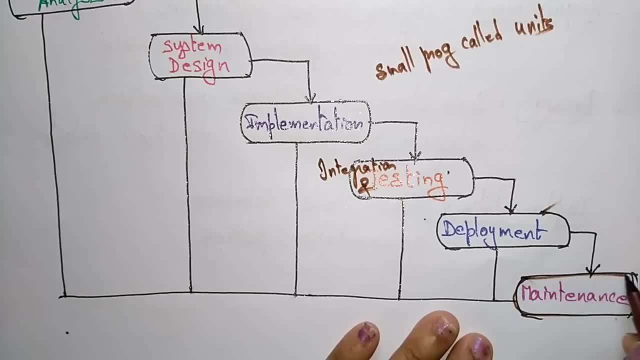 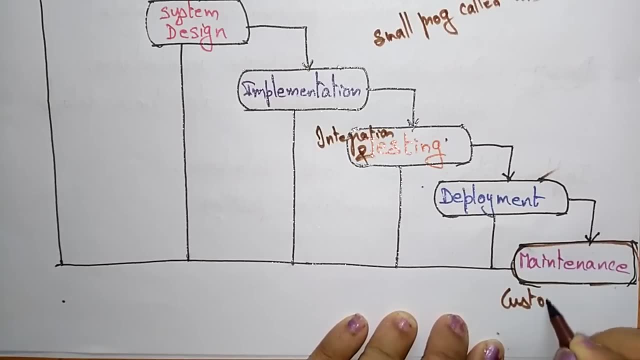 and you have to release again that stage. you call it as a maintenance. so the maintenance stage will be occurred in the customer environment. so the maintenance stage will be occurred in the customer environment, or customer environment only. client or customer environment. so maintenance stage will be done on the customer environment. 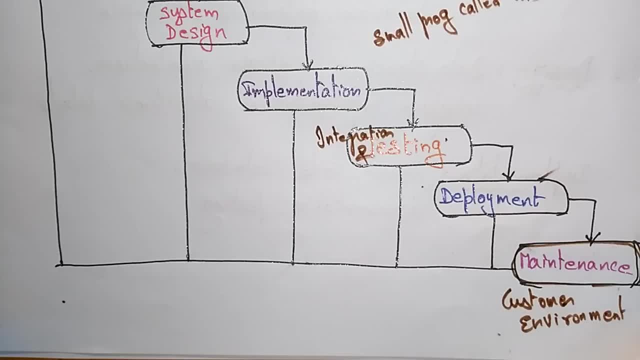 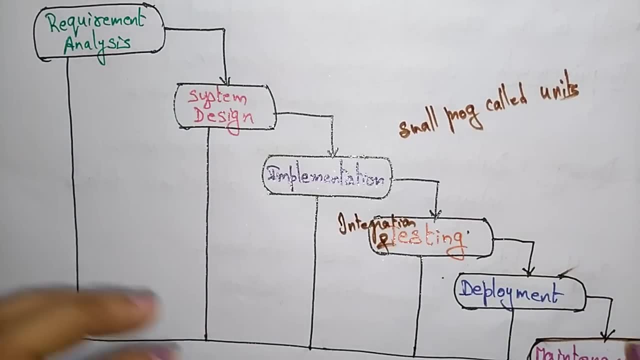 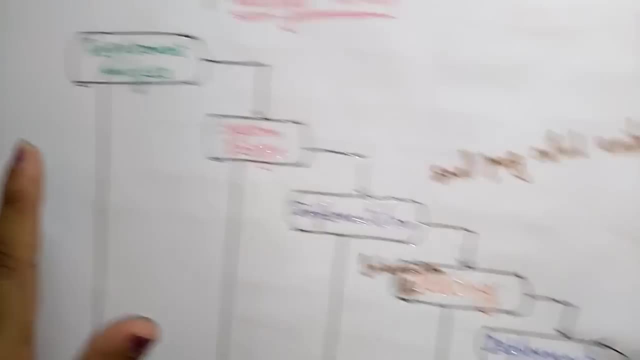 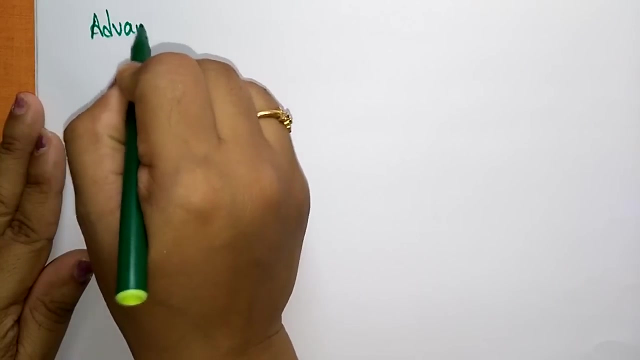 so if you issues comes in the client environment, so those will be fixed as that. you call it as a maintenance. so these are the different stages in the uh waterfall model: first, requirements, system design, implementation, integration and testing, deployment and the maintenance. now let us see the and disadvantages of using the waterfall model advantages. so first thing it is: 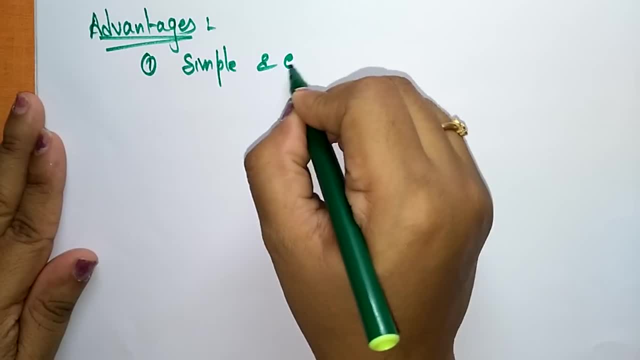 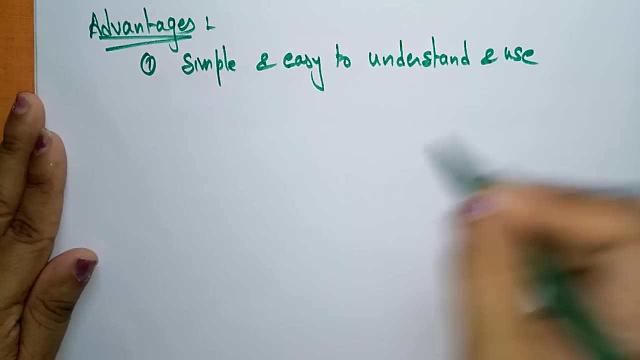 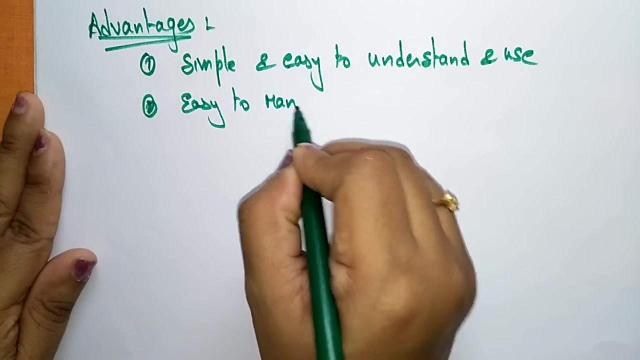 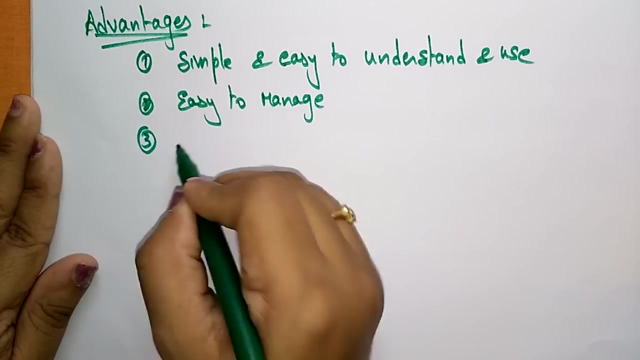 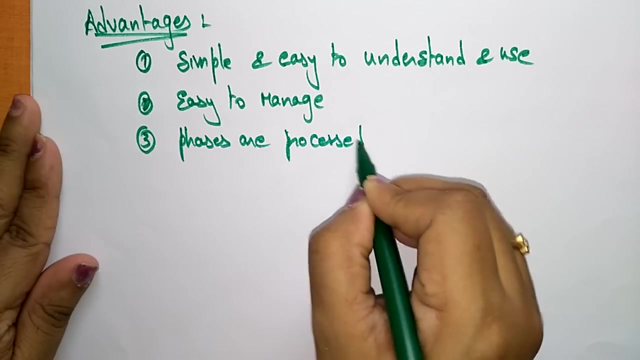 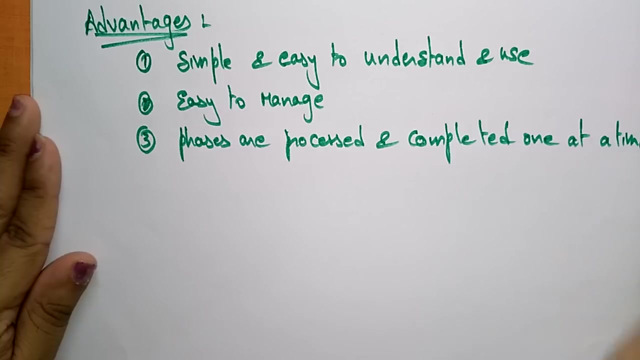 simple and easy to understand and use. okay, and next, it is easy to manage, also easy to manage, and each phase has specific delivery and review for process. next phases, or proceed. phases, or proceed, and completed one at a time, so means once. if if one phase is completed, then only you are supposed to.